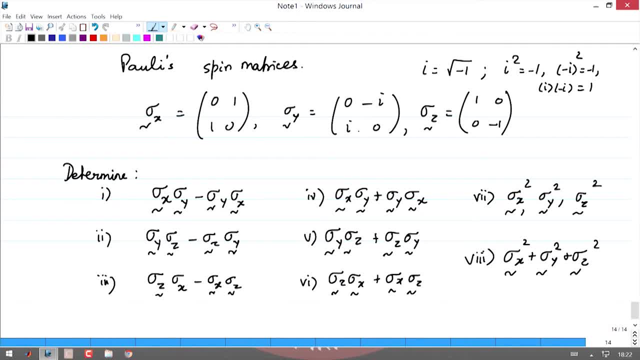 but it has an imaginary quantity, i, and minus i, and i and the imaginary numbers, of course you, you know. So, although the algebra of all the imaginarycomplex numbers, you know, i is defined as the square root of minus 1, and likewise i square, is minus 1, therefore, and likewise minus i, whole square. 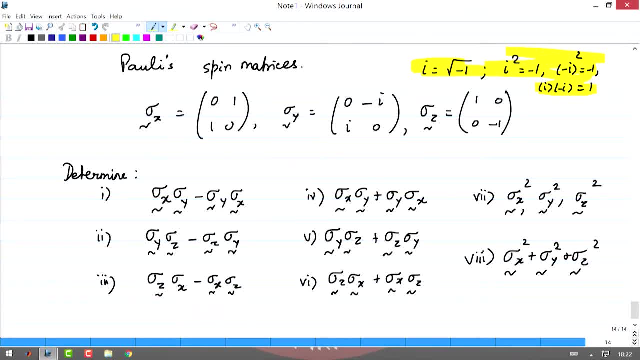 is also minus 1. i into minus. i is 1. ok, Keep that property in my. I mean, keep this in mind. and then you have sigma z, which is the z component of the Pauli spin operator. with 1, 0, 0 minus 1, this is a diagonal matrix, ok. 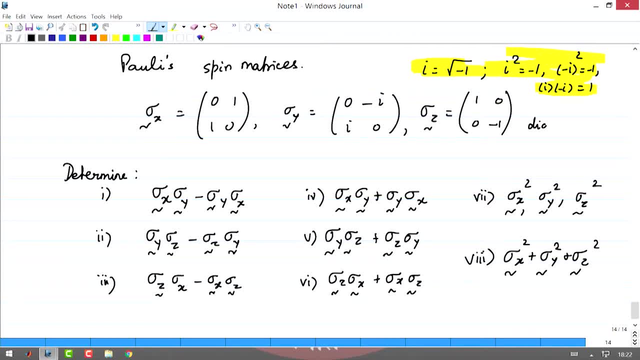 It is a diagonal matrix becauseit has all the off diagonal elements to be 0, it has non 0 elements, only along the diagonal. Now these matrices obey very special properties called anti commutation rulesin the sense that if you take the product of the matrix, 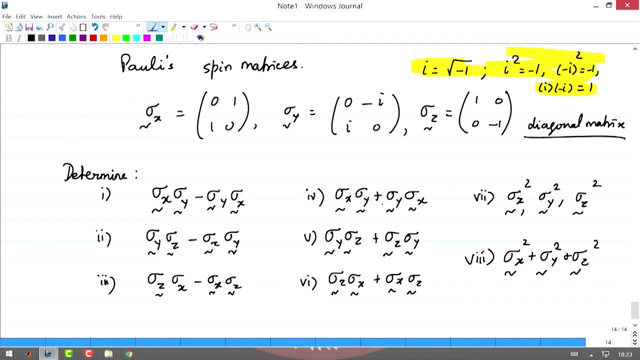 sigma x, sigma y, and then take the commuted products sigma y and sigma x and add them. Find out what answer you get. ok, and there are three such commuter properties which involve x, y, y, x, y, z, z, y, z, x, x, z. So it is sort of cyclical x y, z, ah. So it is like x to y to. 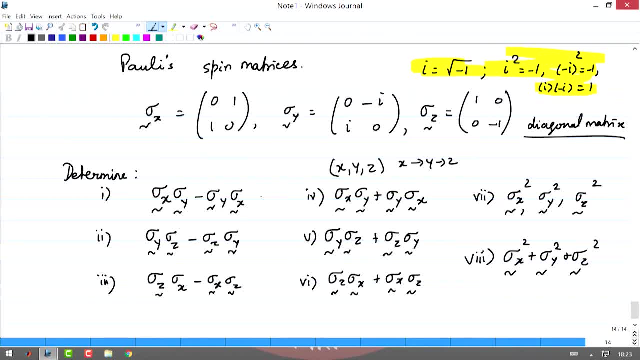 z ok. and if you take the differences between those matrices, you will also find that these matrices do not commute with each other. sigma x does not commute with sigma y. therefore the difference is non-zero. The answer is actually 2: i sigma z ok in this case, and likewise. 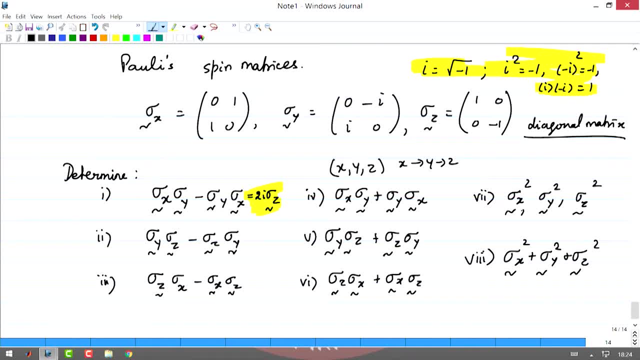 you can find out the other answers. Also, determine sigma x square, sigma y square and sigma z square. you will find out that these are nothing but identity matrices. three times the identity matrix 2 by 2. ok, So these properties are important, therefore, even though 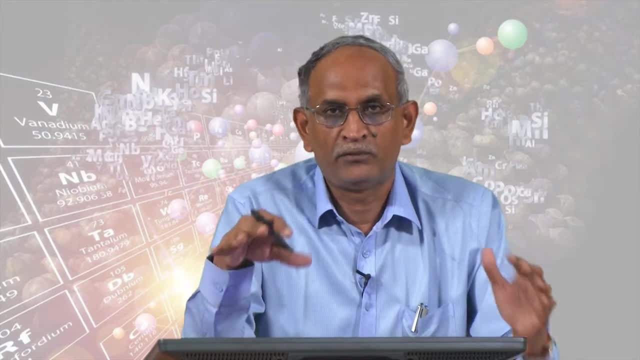 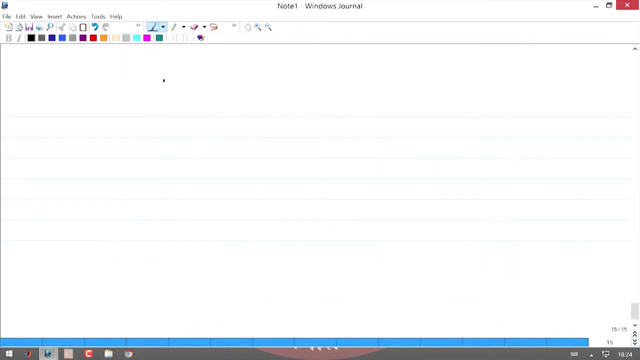 its matrix, multiplication and elementary things. please keep. some of these special matrices will keep coming again and again. ok, Now let us move to the next property of the matrices, particularly the property of a square matrix. ok, A square matrix is one in which the rows and columns of the matrices have the same number. they are 2 by 2,, 3 by 3,, 4. 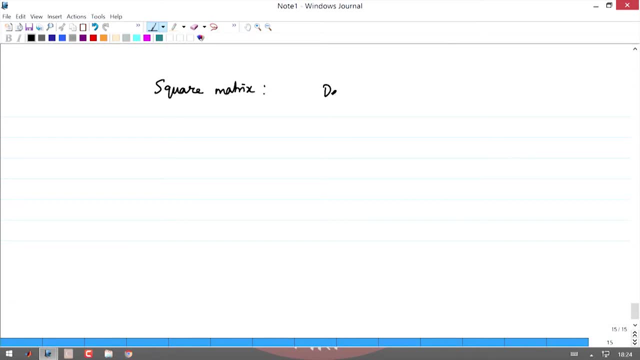 by 4, etcetera. Square matrices can have what are called determinants and the determinant is something you are already familiar with for any array. if you have a, b, c, d as a matrix, determinant is written by the symbol and that is a d minus b c, which is a number. ok. 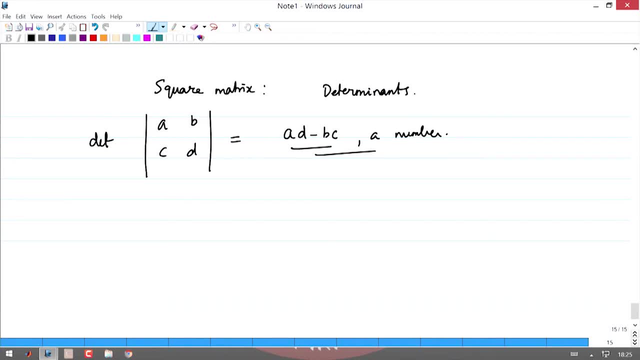 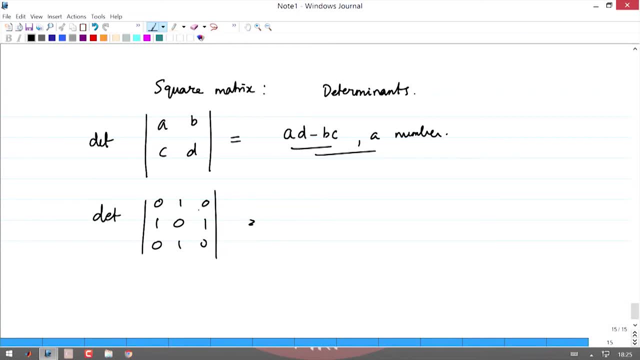 mathematics that you studied that you can expand the determinant along any given row or along any given column. So let us expand this along the first row. if we do that, it is 0 times the. if you do 0, then it is the cofactor of 0 is 0, 1, which is which is called. 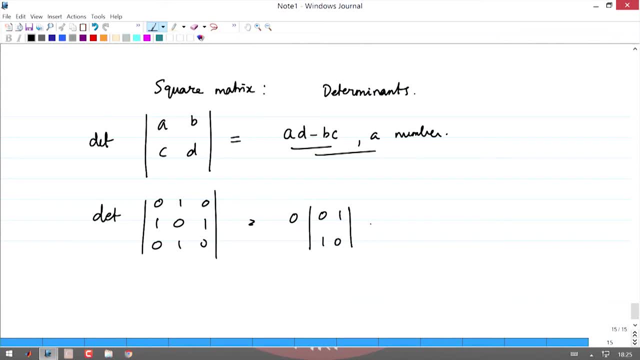 the minor: 0, 1, 1, 0. And since you go to the second element, the, So you can see that the determinant of a, the sum of the indices row plus column index, is odd. this will be a minus sign and you will. 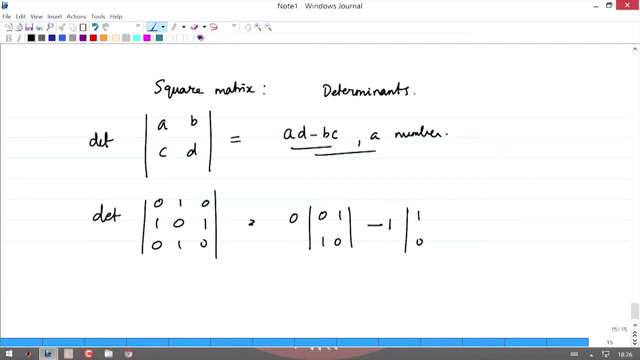 see that it is 1 times 1, 0, 1, 0 and the last one is 0 times 1, 0, 0, 1. So if you take any element, 0, for example, then all you would do is in doing the matrix multiplication you. 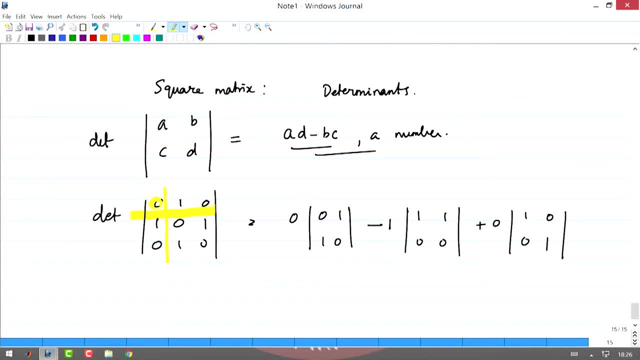 will delete that row and you will delete that column, And so the rest of it is 0 1 1 0, which is what is here? ok, And in the same way, the minor of 1 will be deleting, deleting this column and this row. So what is left over? issorry, not this one. So this is 0 1 1 0. 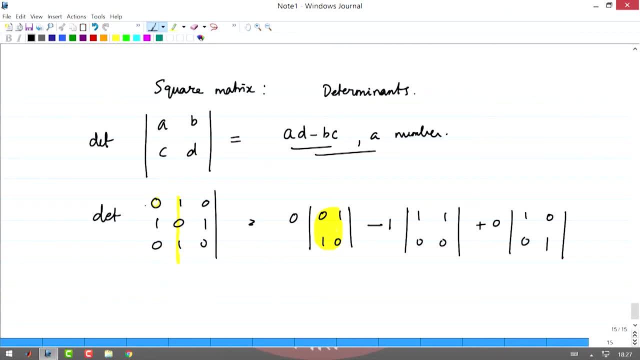 1 0, 1, 1 0. So this is 0 1 1, 0, 0, 1 0, which is what it is. it is 0 1 1, 1 0, exactly this. So the rest of it is 0, 1 1, 1, 0, 0, 0. In determining the minor of 1, you will delete this column. 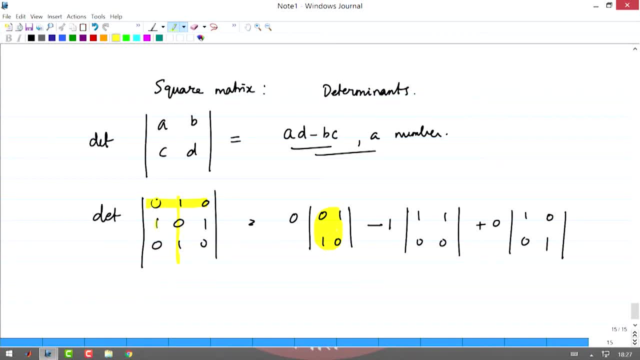 and this row. So what is left over is 1 0, 1 0, which is what is here. Of course, the answer for this is 0. ok, If you do a matrix such as this- 0 0, 1 0- then 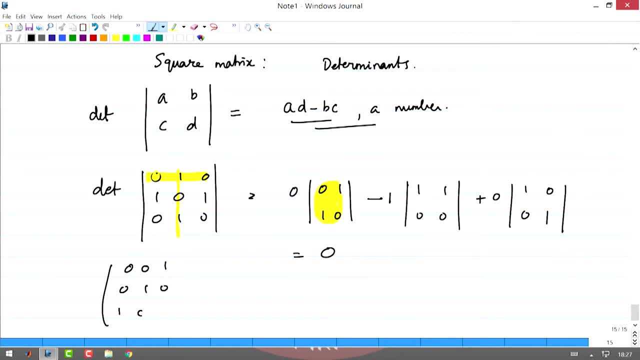 you are getting a code, So you have to do the same thing, but you have to do the new 1 0, 1 0, 1 0 0.. If you want to calculate the determinant of this matrix, then it is clear. 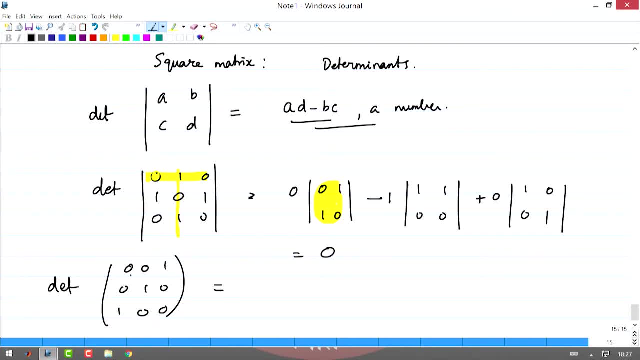 that the first two are 0. So you do not need them, and the last one is plus 1 times whatever is the minor, and the minor is minus 1.. So the determinant of this matrix is minus 1 and you can also verify that the determinant of A B- C is the determinant of A B times C. 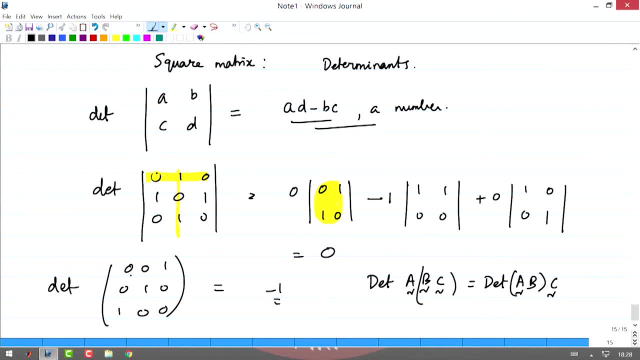 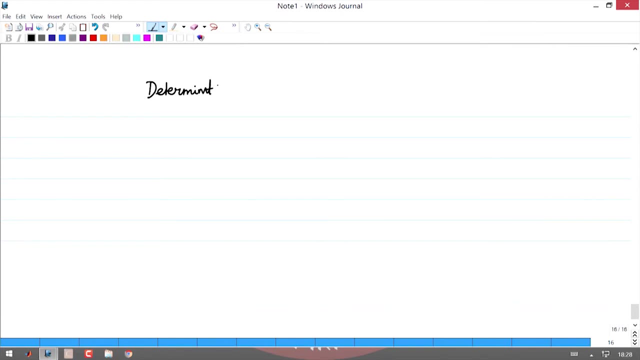 because you know that matrices obey the associativity. determinant of is alsoit also follows the same properties. ok, Now there are matrices for which the determinant is 0. And these are called the singular matrices. The singular matrices are such that if you want to define an inverse for the matrix A, suppose you have a matrix A, B, C, D and an inverse. 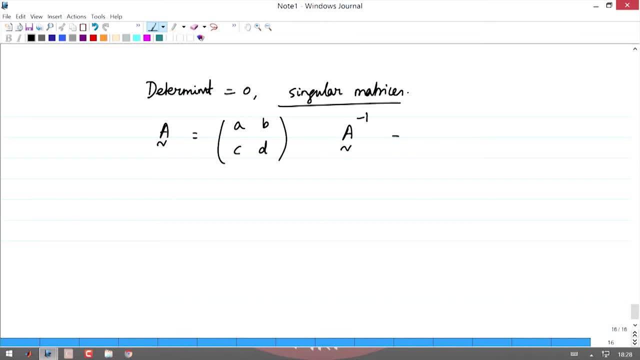 is to be defined A inverse. The property of the inverse is that A times A inverse is the identity matrix and it is the same thing as A inverse and A, So in that sense they commute. ok, This is the property of the inverse. Therefore, if A is of A, B, C, D and you want 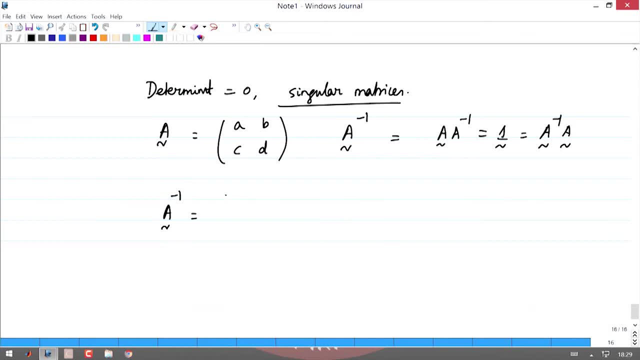 to calculate A inverse. ok, and let us write this as P, Q or S. then AA inverse would be A, B, C, D, P, Q, R, S, and that should give me the identity matrix, namely 1, 0, 0, 1, and since this is a, 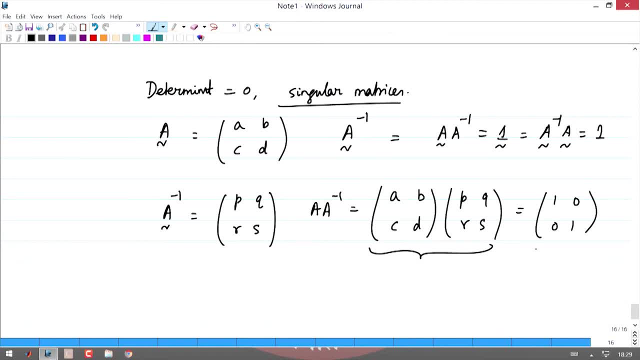 matrix. the elements of this matrix should be the same as the elements of this matrix, So let us calculate them. it is A? P plus B R. that is the firstrow first column. then the first row second column is A? Q plus B S. likewise C? P plus D R and C? Q plus D S. this should be. 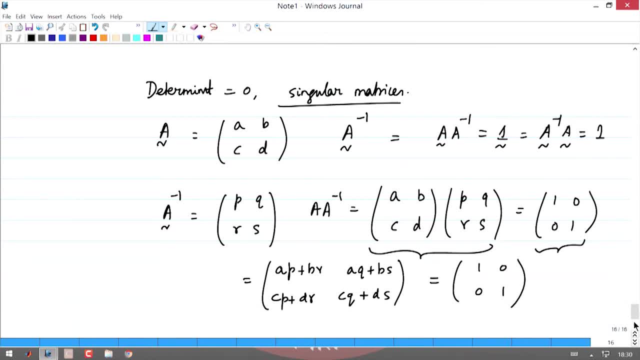 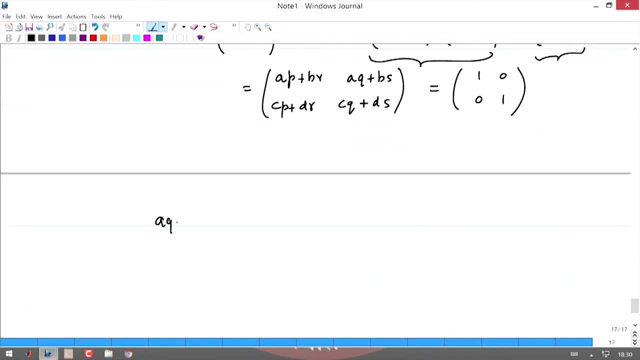 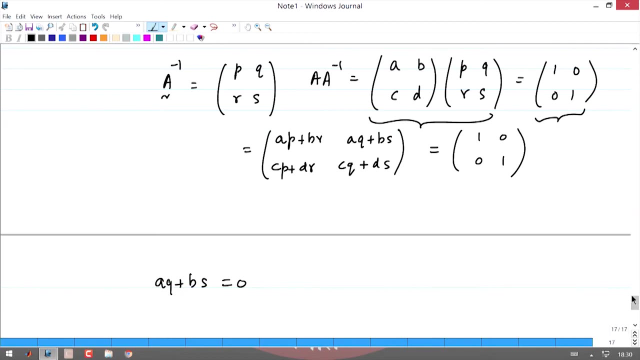 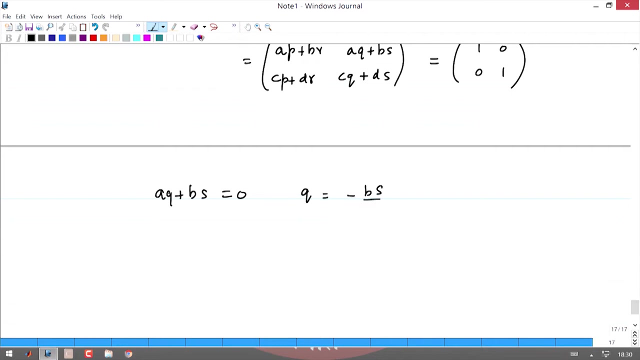 1, 0, 0, 1. given this, you can immediately see that the element A, Q plus B S is 0, and since we are interested in finding out P, Q, R S In terms of A, B, C, D, which we know, so we can write: Q is equal to minus B S by A, and likewise. 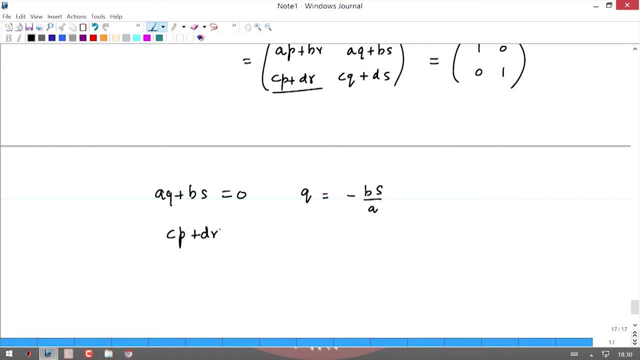 this element, C P plus D R is equal to 0, and so I will write: P is equal to minus D R by C. We also have the property that A P plus B R is equal to 1.. And since we are interested in finding out, Q is equal to minus B S by A, and likewise. 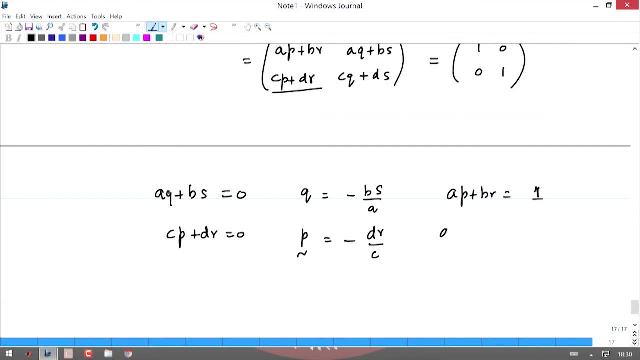 we know that P is minus D R. you have A times minus D R by C plus B, R is equal to 1. So this gives you immediately minus A D plus B C times R is equal to C. So what is R? 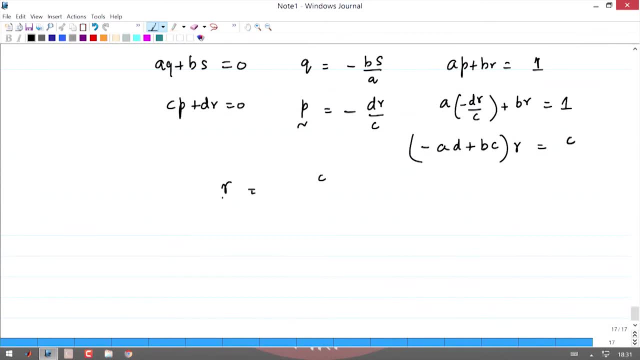 R is C. So this gives you immediately minus A D by B C minus A D. And once you know R, you can immediately findhere. Since R is connected to P, you can immediately find P. therefore you determine P, you determinesimilarly. 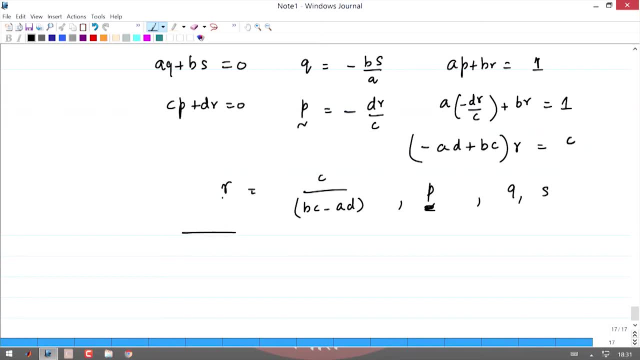 Q and you determine S. ok, What is the final answer? So the final answer will turn out to be 1 by A, D minus B C times. The final answer is 1 by A D minus B C times the matrix D minus B minus C A. It is easy. 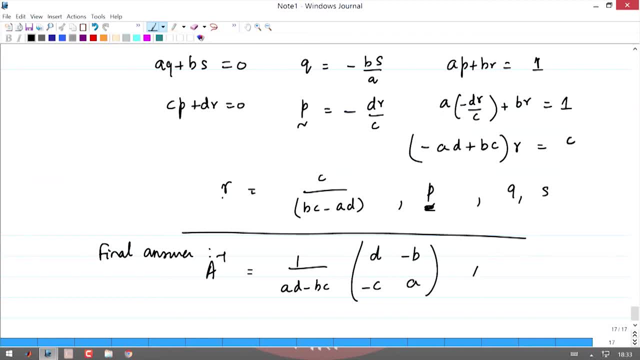 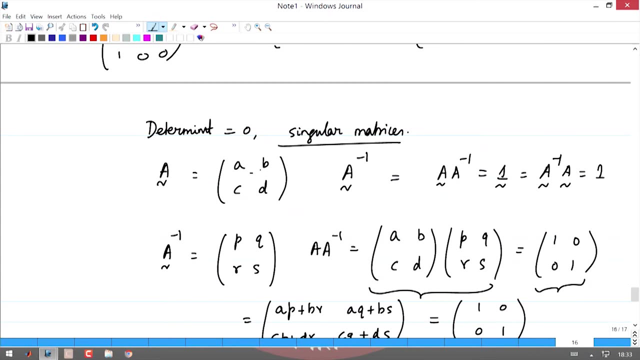 to verify that. if this is A inverse, then A into A inverse actually gives you the matrix 1 0 0, 1. ok, Now what is important is this factor A D minus B C. Please note that A D minus B C for this matrix is nothing but the determinant of A. Therefore it should. 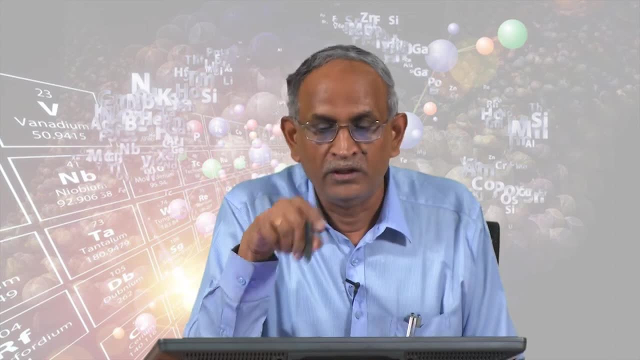 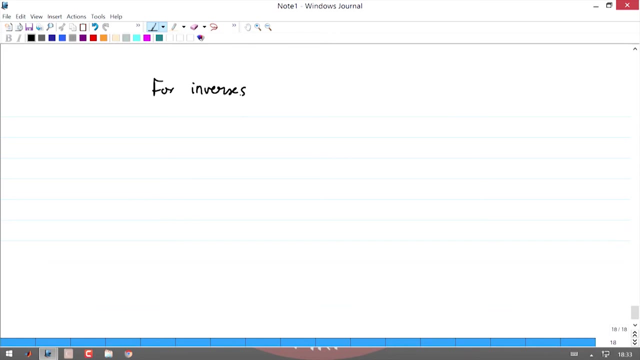 not be 0. Therefore, for inverse to exist, the matrix should be non singular. for inverses of a square of square, matrices determinant should not be 0. matrix should be non singular. ok, In my lecture notes, of course, I will give you a very clear formula for inverses of a. 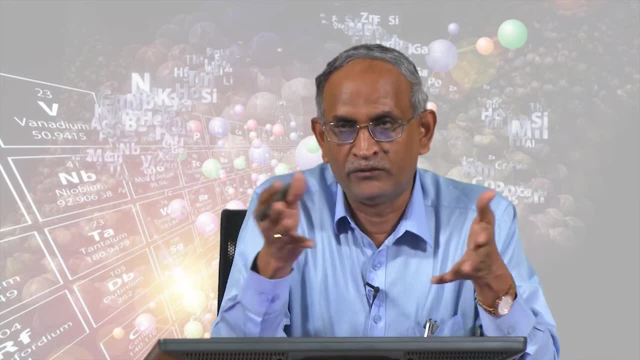 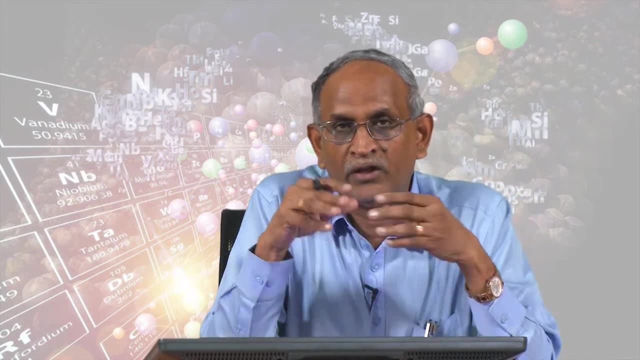 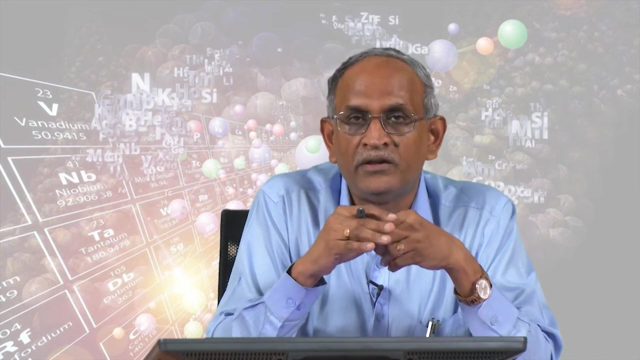 general matrix in terms of what are known as the determinant as well as the cofactors of each elements. but here we have seen that, So likewise, it is easy tocalculate inverses, and inverses are very importantwherever they exist. theit is important to find to the inverse. 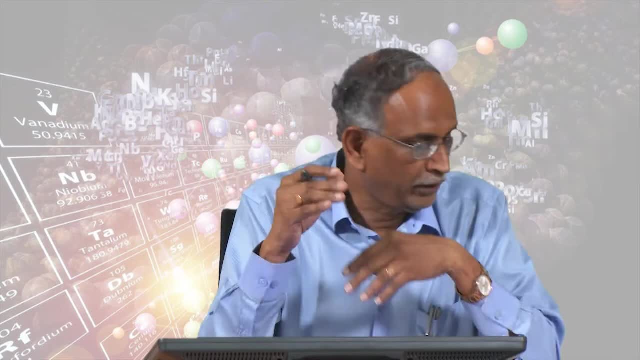 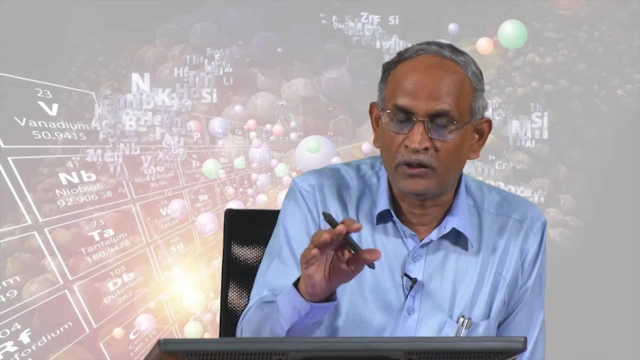 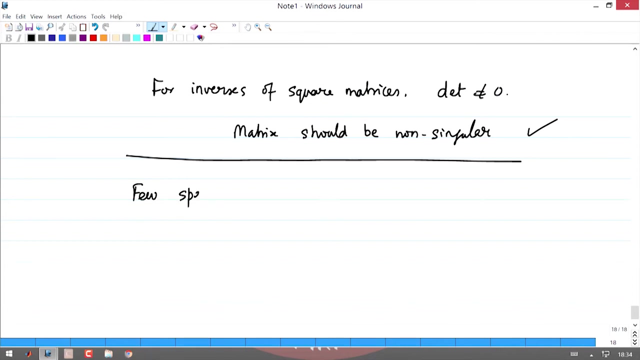 and associate the properties of the inverse with certain types of matrices. In the next and the finalthe part of this particular lecture, I shall introduce you a few special matrices in which inverse will have a critical role. ok Now, your matrix is a symmetric matrix If the element a, i, j, 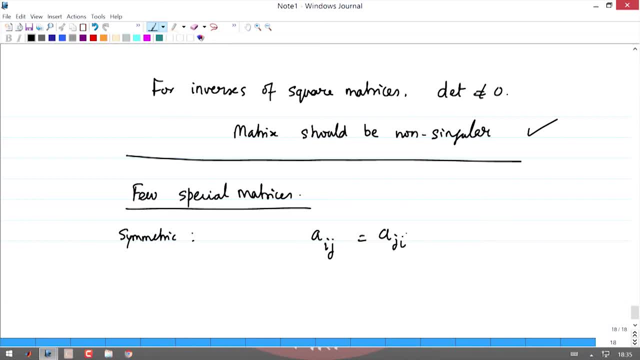 i. j is the same as the element j, i. that means n- i. why s a? It is decided that anywhere where n i exit from r a, 1 is shrimp, is a small function somehowiele, or instead there will be any invariant. 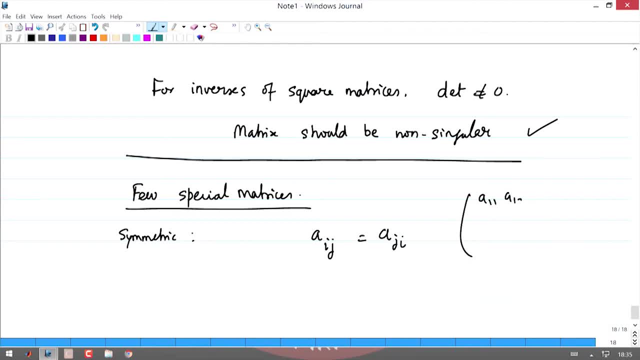 the matrix: a 1: 1, a 1- 2, a 1: 3, a 2: 1, a 2: 2, a 2: 3, a 3: 1, a 3: 2, a 3: 3.. If you write: 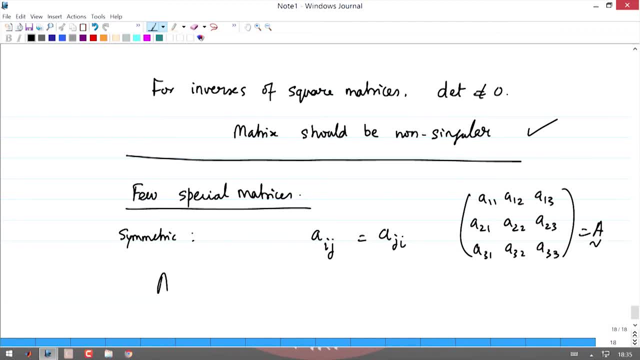 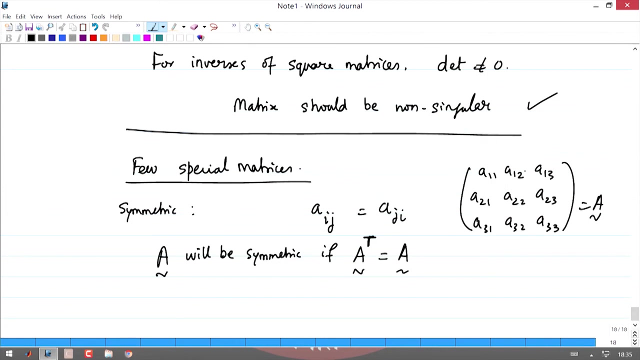 this as a matrix. this a will be symmetric if: if the transpose of the matrix, which is obtained by transposing the rows and columns of any given matrix is equal to the matrix itself. Therefore, a is symmetric. if you have a 1- 2 and a 2, 1 are the same, a 2- 1 likewise. 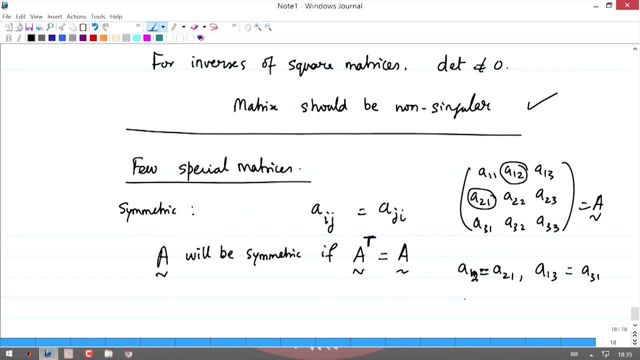 a 1, 3 and a 3- 1 are the same and a 2, 3 and a 3- 2 are the same. That is also easy to see because the transpose of this matrix is: a 1, 2 and a 3, 2 are the same and a 2, 3 and a. 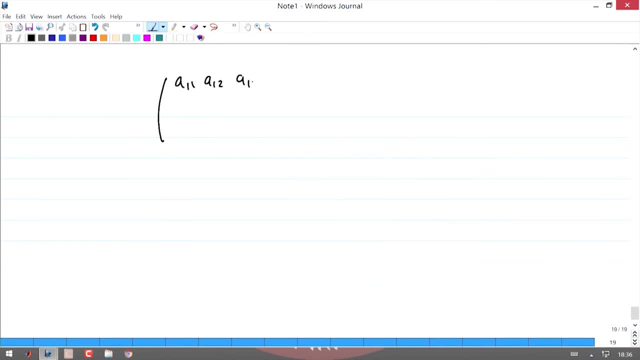 3- 2 are the same. that is also easy to see because the transpose of this matrix is: a 1- 1, a 1- 2, a 1- 3, a 2- 1, a 2- 2, a 2- 3, a 3- 1, a 3- 2, a 3- 3.. If you take the transpose, 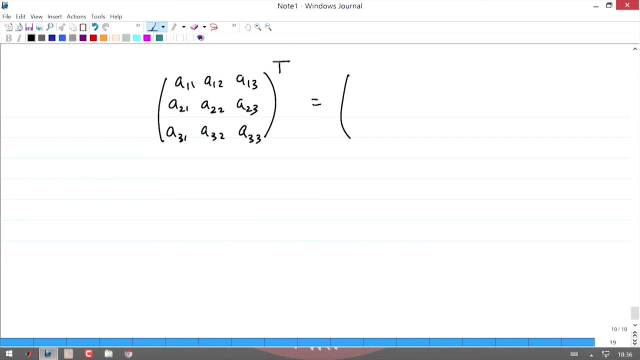 of this matrix. you are basically transposing thiscolumn into a row or this row into a column. So let us take this row, then it becomes the first row, becomes the first column: a 1- 3, a 1- 2, a 2- 3. and the third row: a 3- 1, a 3- 2, a 3- 3. ok, If this were to be equal to the. 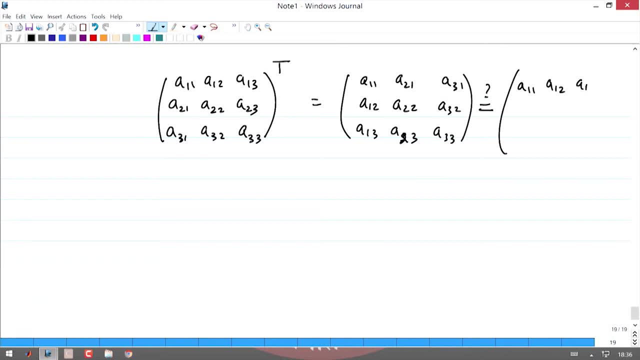 original matrix: a 1: 1, a 1, 2, a 1, 3, 2, 1, a 2, 2, a 2, 3, a 3: 1, a 3, 2, a 3, 3,. then you: 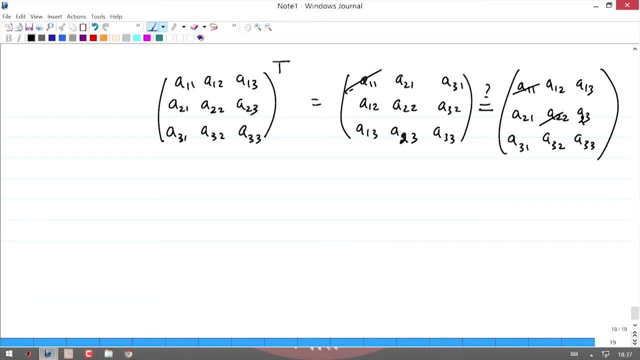 see that there is no problem with the diagonal elements because they don'ttranspose themselves. So this is the first row and the second row of the matrix. So a 2- 1 should be a 1- 2 and a 3- 1 should be a 1- 3 and a 2- 3 should. 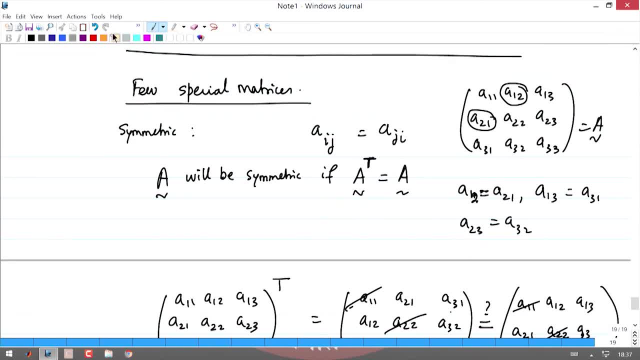 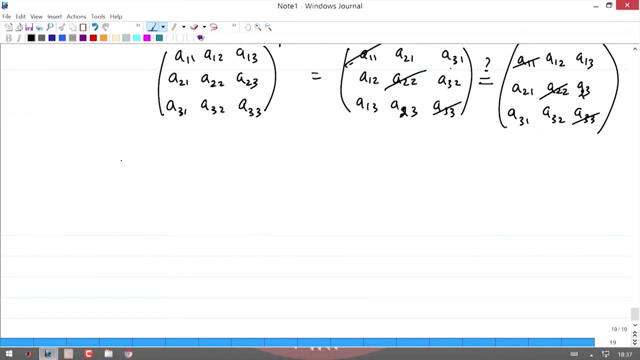 be a, 3, 2, which is what I have written here. ok, So this is required if a t is equal to a. Now, this is for symmetric matrices. Now, if the elements are complex, you would see that we can define in a similar way. 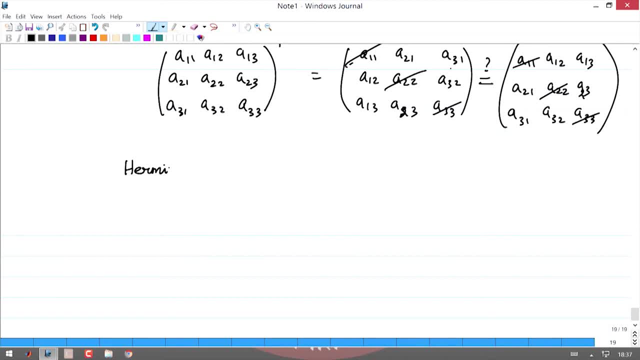 way what is called the Hermitian adjoint. The Hermitian adjoint of any matrix A is denoted by: of any A is denoted by the symbol A dagger, ok. And if the matrix of A is denoted by the elements A, ij, then A dagger is the elements of the matrix A transpose star. 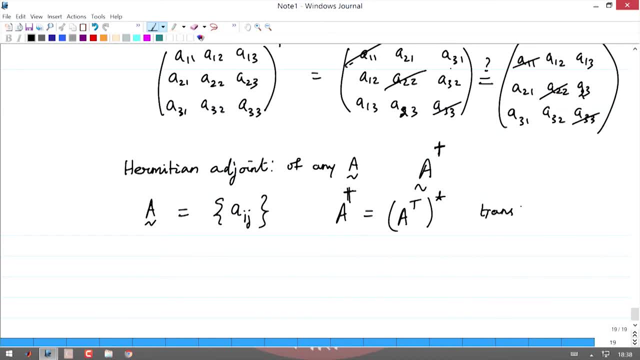 Transposed complex conjugate. Therefore, if you write A dagger, ij is A, j i star. ok, The matrix is transposed and its complex conjugate. This is the element. This is defined as a Hermitian adjoint of A. It does not tell you. 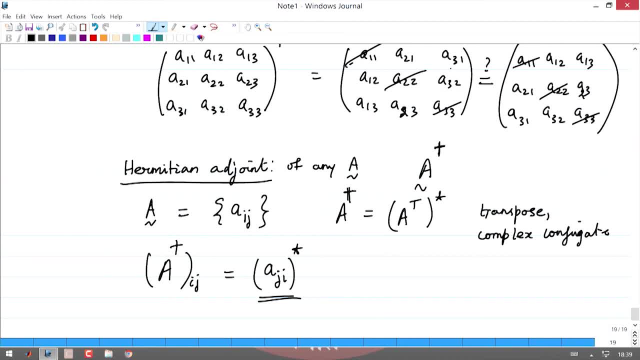 anything about whether A is the same as Hermitian adjoint of A dagger, that is, A is equal to A dagger. It does not tell you anything that For every matrix A we can define a Hermitian adjoint. If the element is real, then the Hermitian adjoint is given by the transpose. 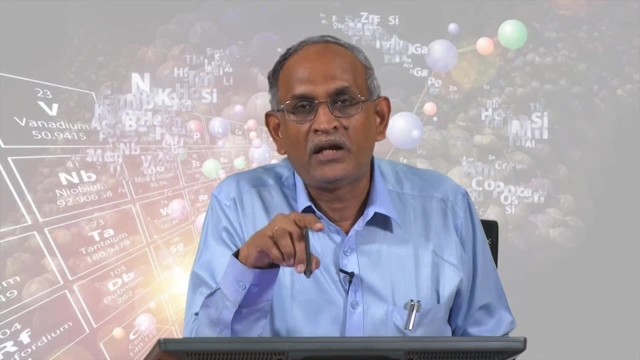 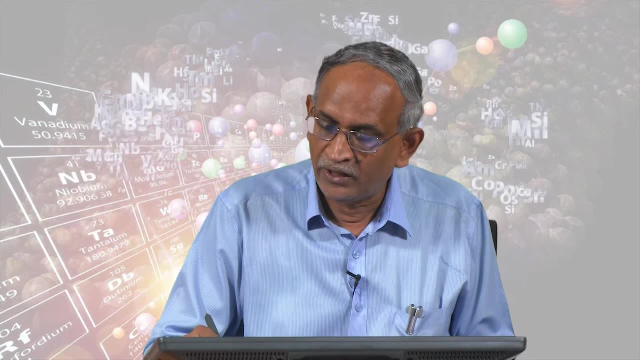 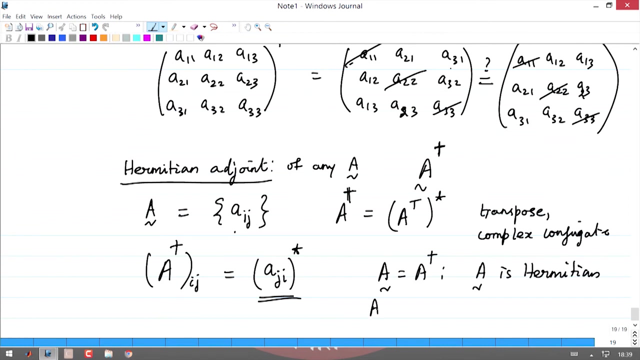 of the matrix, the elements of the transpose of the matrix. A matrix is Hermitian only if a is equal to a dagger, then we say a is Hermitian. In the same way we say when a is equal to a of t, we say a is symmetric. So the Hermitian includes complex numbers and 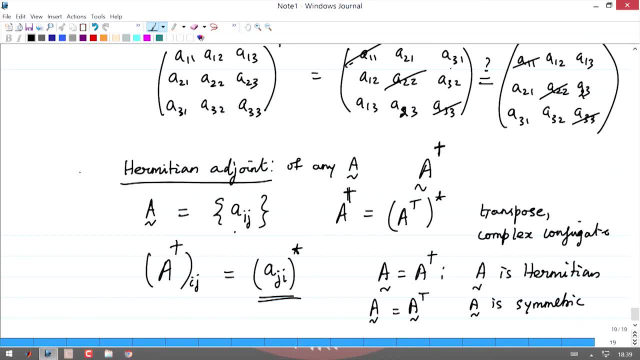 therefore, the complex conjugation is important in the definition Hermitian adjoint and Hermitian matrices, that is, in matrices for which the matrix and its Hermitian adjoint are equal. they are fundamentally important. In fact, all observable quantities in quantum mechanics. 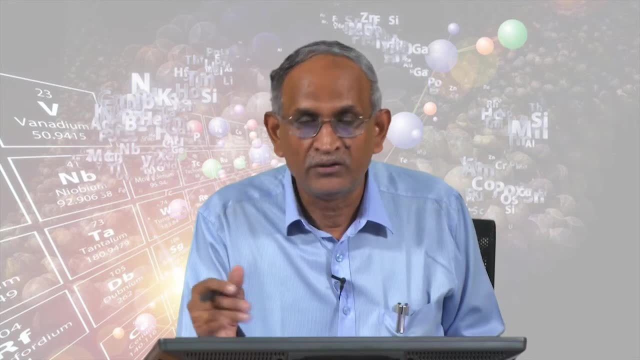 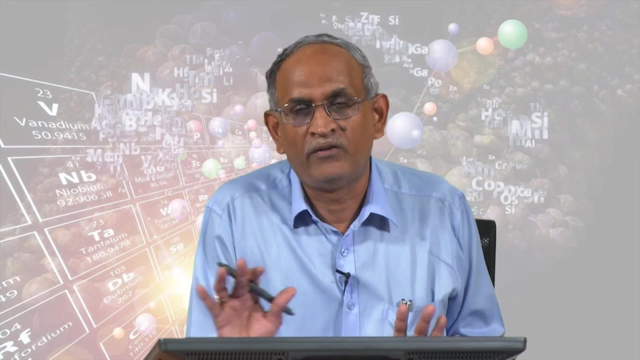 in the matrix formulation are represented by Hermitian matrices. Actually, in mathematical parlance it is. they are represented by what are known as the self adjoint matrices. but for our course, if we keep the terminology simple, and Hermitian matrices are very, very- 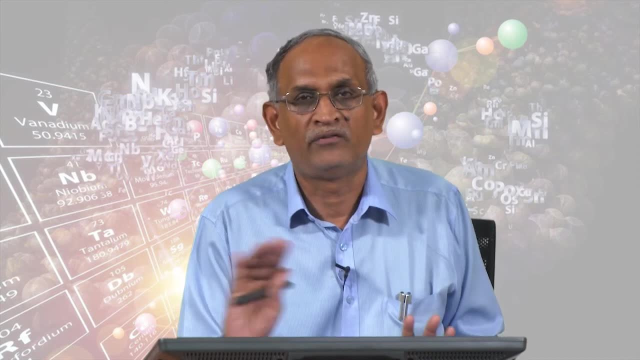 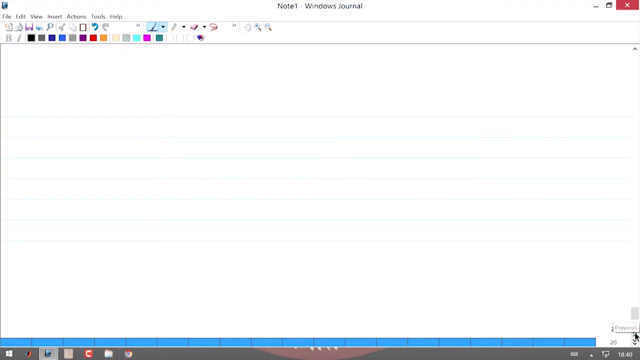 important. in quantum mechanics All eigenvalues are eigenvalues, So they are the eigenvalues of Hermitian matrices that we willeventually find then. the other important property of A matrix, other important type of a matrix, is known as orthogonal type. ok A matrix is orthogonal if ok a is orthogonal. 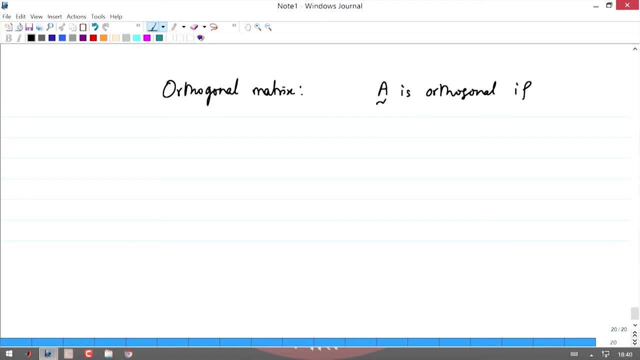 if a- t, the transpose of A is equal to the inverse of A, that is, A A inverse. if it is 1, then it is the same thing as saying A A t is equal to 1.. Since clearly inverse is involved, the determinant of A should not be 0. A is not 0. In fact it will turn out to be 1. So 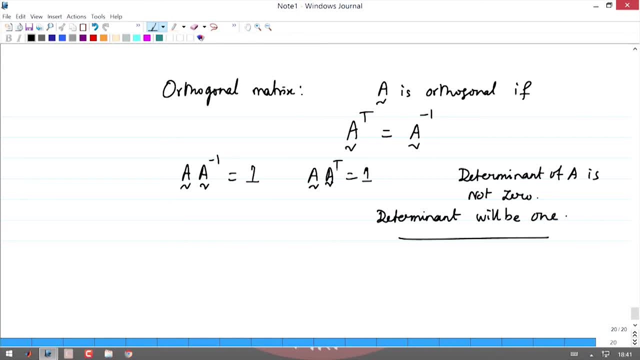 because 1 involves a determinant of A, A, a. t involves a determinant of A in the denominator denominator. Therefore, you would see that orthogonal matrices are matrices for which the transpose of the matrix is equal to the inverse of the matrix, or you compute inverse. 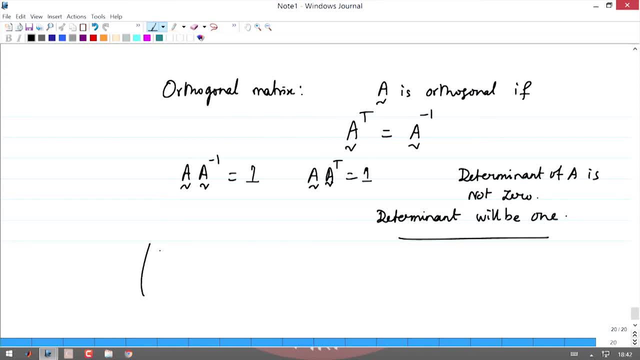 by simply transposing the matrix. So if I have a matrix like cos theta, sin theta minus sin theta cos theta, then I know that the determinant of this matrix is 1 its cos square theta plus sin square theta, minus of minus sin square theta And the. this matrix is orthogonal. 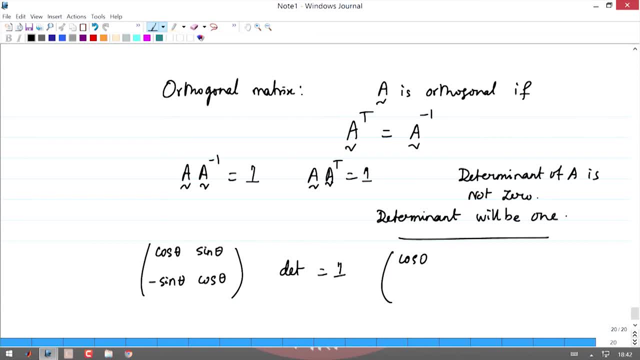 its inverse is the transpose, namely cos theta minus sin theta, the first column becomes the first row and the second column is the second row. sin theta, cos theta is a inverse, if this is a ok, and this is nothing but the transpose of the matrix. So here is a very simple example for what. 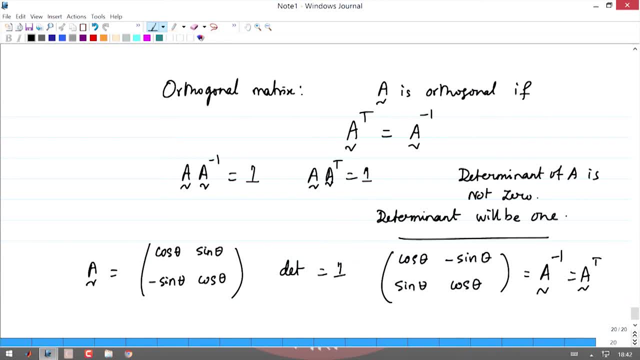 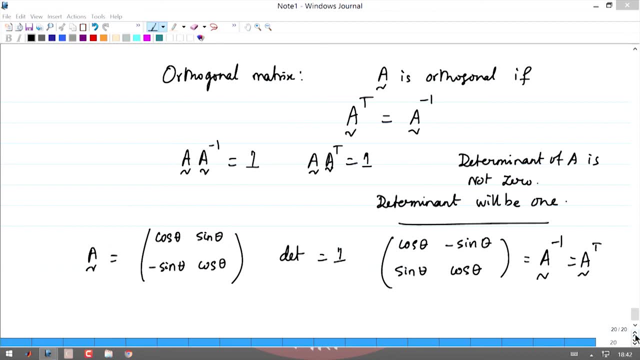 is known as a transpose of the matrix. So here is a very simple example for what is known as a transpose and the inverse. these are for real elements. If you have complex elements, then one does not define an inverse in this way or theorthogonal in this manner. 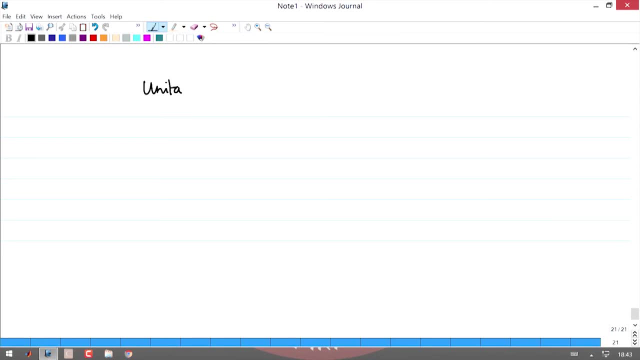 but one defines what is known as a unitary matrix. a unitary matrix, u, is unitary if u is equal to u dagger. the Hermitian adjoint, u, is not Hermitian, that is, u is not equal to u dagger. in general, ok, no, Therefore the inverse of the matrix is the. 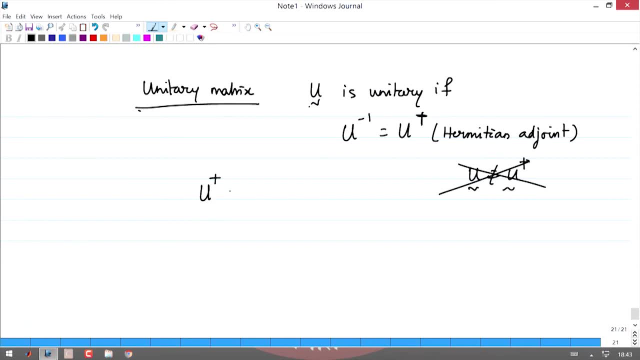 same as u dagger, So u dagger is, of course you know. is u j i star? ok, u i u dagger. is u dagger, i j. is u j i star. the rows and columns are immersed in I mean transpose and complex conjugate. Therefore, this is the same as the u inverse i j, So the property is u. 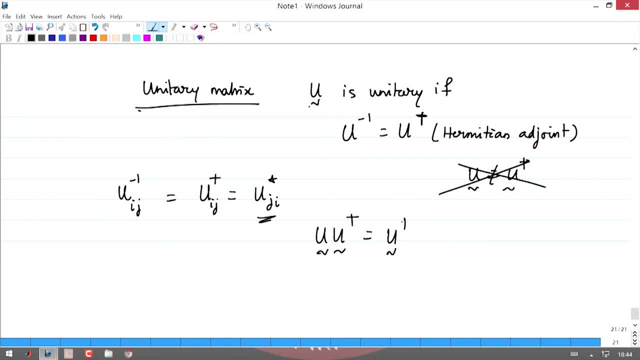 u dagger, which is the same as u dagger u, and that is equal to 1. ok, Obviously, all are square matrices. we are not talking about any other at this point. ok, So this is the. this is the identity matrix. Therefore, if u is n by n, this will be n, an identity matrix. 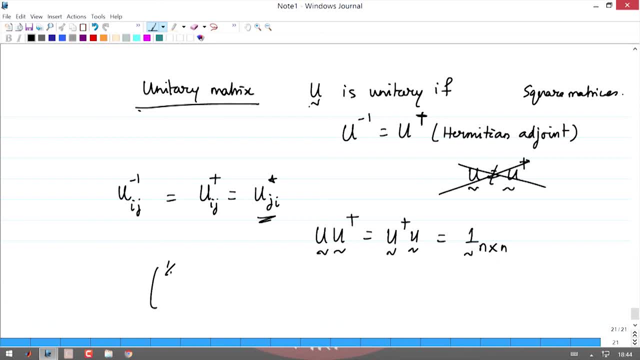 of n by n. What is the example of a unitary matrix? very simple: 1 by root 2, 1 by root 2. let me do i by root 2, ok, and then I write 1 by root 2 minus i by root 2. If I take this matrix, then its inverse. if this is u, its inverse. 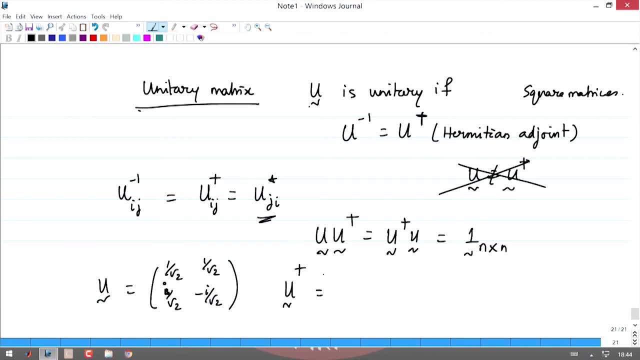 is u dagger and u dagger is the transpose of the matrix 1 by root 2, i by root 2, but also complex conjugate. Therefore i becomes minus i, for the first column becomes the first row and the second is 1 by root 2. i minus i by root 2, which becomes plus i by root 2. 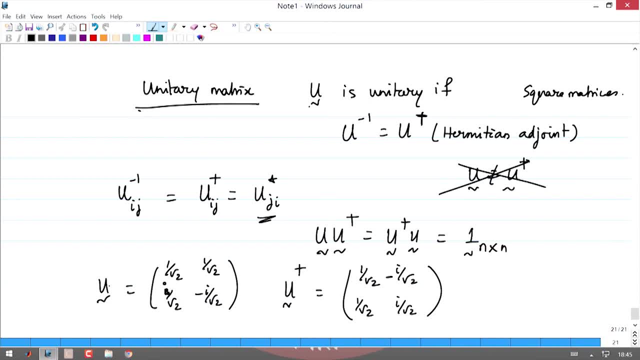 ok, If you multiply these two matrices, you will see u u dagger is 1 by root 2 times 1 by root 2 plus this, So that is 1, and the secondcolumn is minus i by root 2. this i by that is also 0, and likewise. 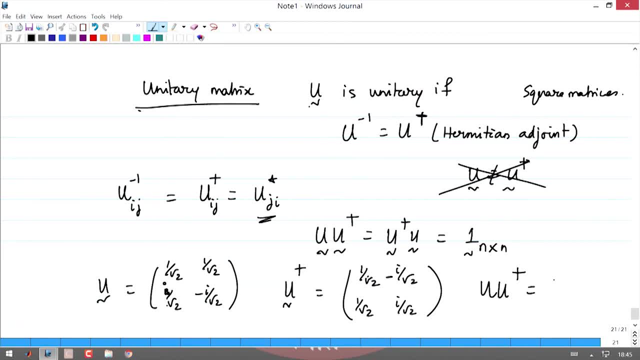 this is 0. So this is u? u dagger is 1 0 0, 1. So this is an example. a very simple example of a unitary matrix in two dimensions is given Now what I have not said. in conclusionI should state that orthogonal also means the following: 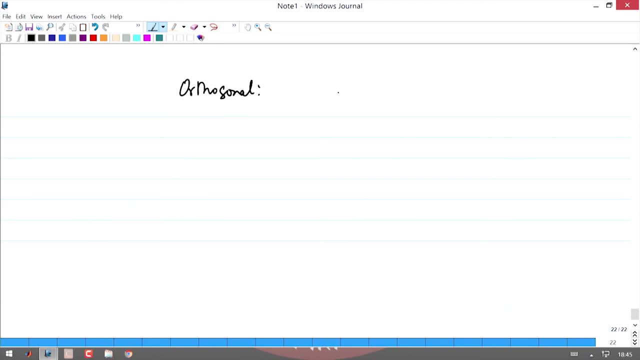 Orthogonal matrices have columns and rows which are orthogonal to each other or orthogonal to each other and are normalized. So if I take a matrix, a as orthogonal, then the property of this column A 1- 1, A 1- 2, A 2- 1, A 2, 2.. Please remember the determinant is 1, which is A 1, 1 minus. 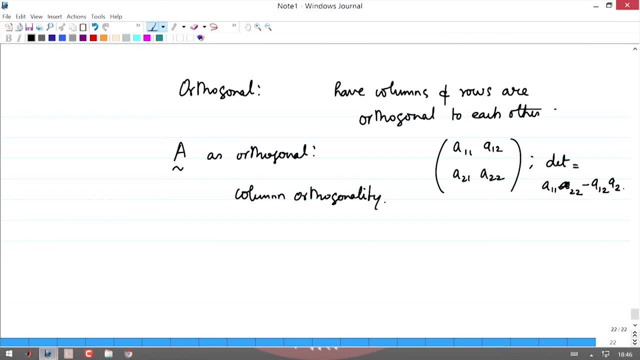 A 2- 2 minus A 1 2. A 2- 1, this is 1 and the column orthogonality essentially means column 1 multiplied element by element within column 2 will give you the answer 0. A 1 1, A 1- 2. 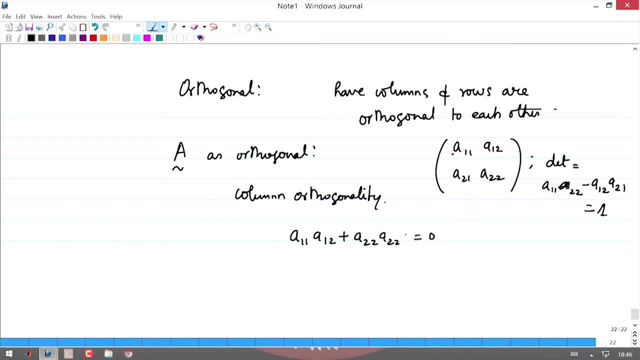 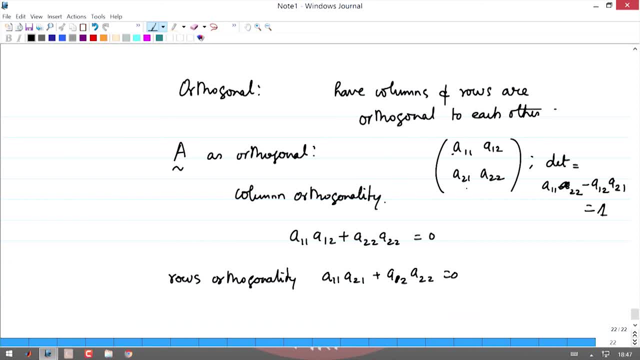 A 2, 2, that is 0.. What about rows by themselves? A 1: 1 square plus A 2: 1 square, that will be 1, and likewise A 1, 2 square plus A 2: 2 square will be 1. So the rows and columns are normalized. 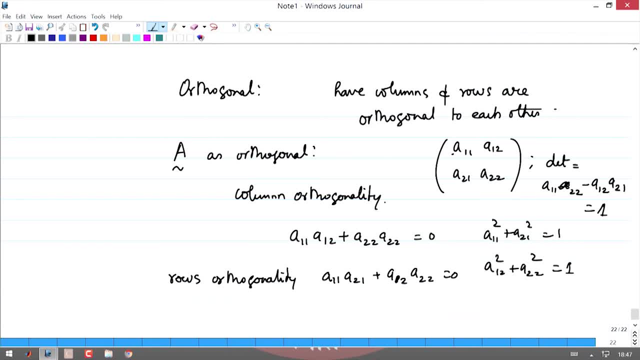 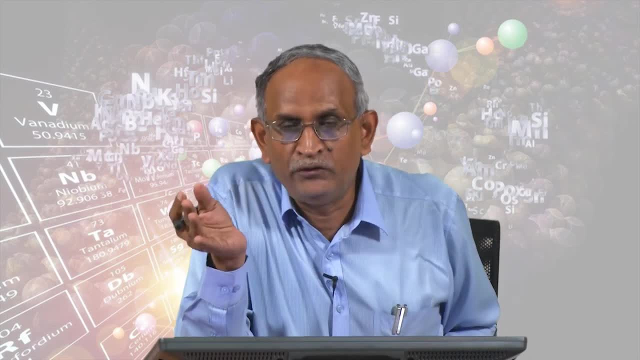 and the rows and columns are orthogonal to each other. this is for an orthogonal matrix. For a unitary matrix, one of the rows that we take in the product of two rows has to be the complex conjugate of the row itself. And therefore, when you say unitary matrix, 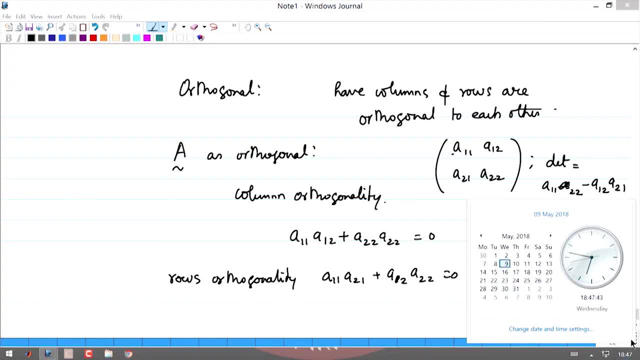 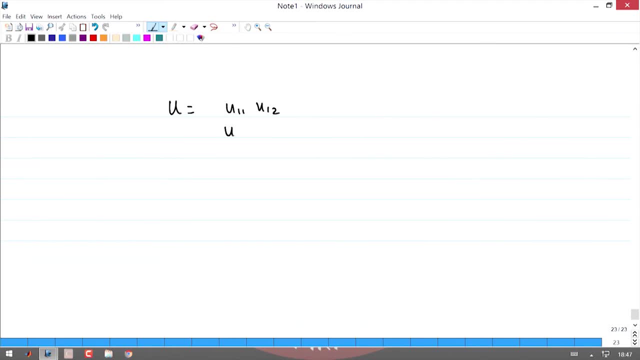 you suppose you write to the matrixu as u 1 1, u 1 2, u 2 1, u 2 2. as a simple example, then the column orthogonality essentially means column 1 is orthogonal to column 2.. 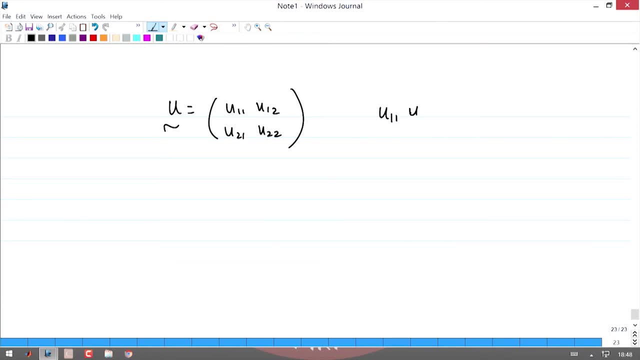 So you either take column 1, real, but then you multiply with the complex conjugate of column 2 plus u 2, 1, u 2, 2 star, that is 0.. So this column multiplied by the complex conjugate of this column is 0. it does not. 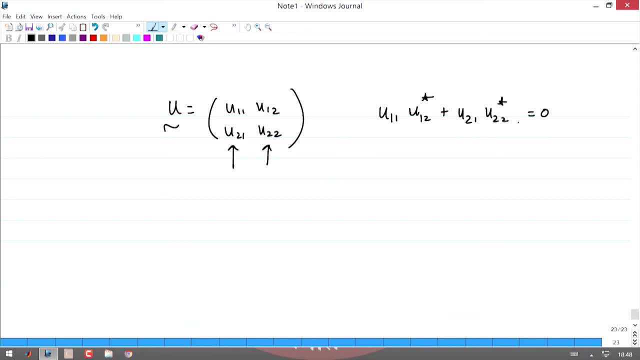 matter which one is taken as a complex conjugate, because if a number is 0, its complex conjugate is also 0. So if you take this row, this column, and you take the complex conjugate of it, it is still 0.. The other thing is the orthogonal. the normalization essentially means: 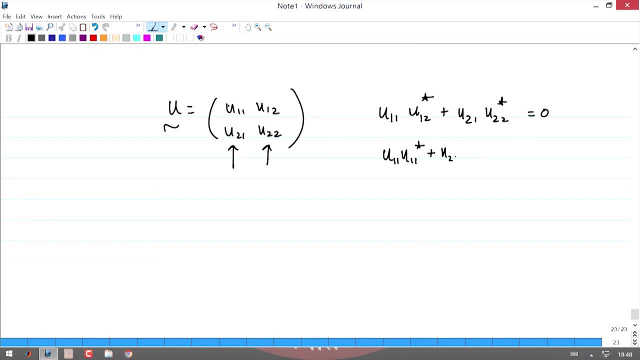 u 1: 1, u 1: 1 star plus u 2: 1, u 2: 1 star, that is equal to 1.. Therefore, unitary matrices are such that the rows and columns are normalized and the rows and columns are orthogonal. but